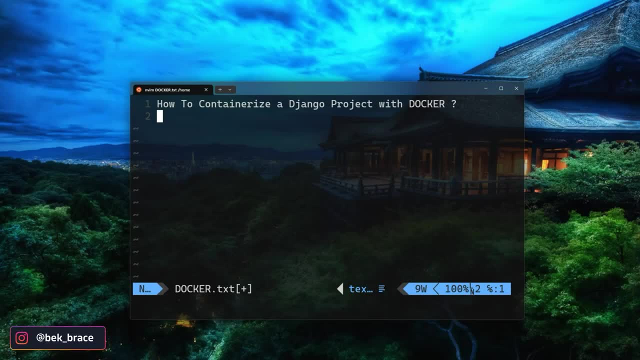 Hey, what's going on everyone? this is Begbrace channel, your go-to place where we explore all things programming. My name is Emir and in this video we're going to check out how we can containerize a Django project using Docker. And if you're new to the channel, I would like to 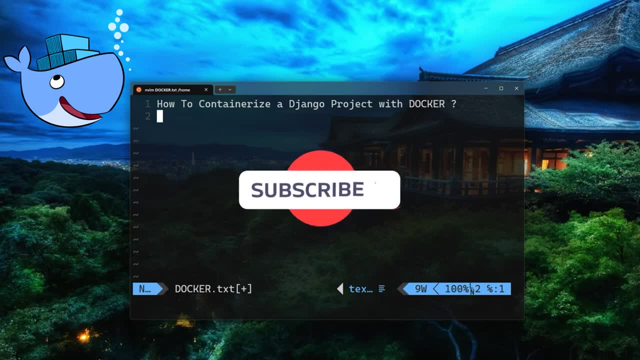 welcome you and I would like also to ask you to hit that subscribe button. Also hit that notification bell in order to get the latest updates and videos from our channel. Now, before we get started, let me clarify that this video is not new. It's actually part of our older video. 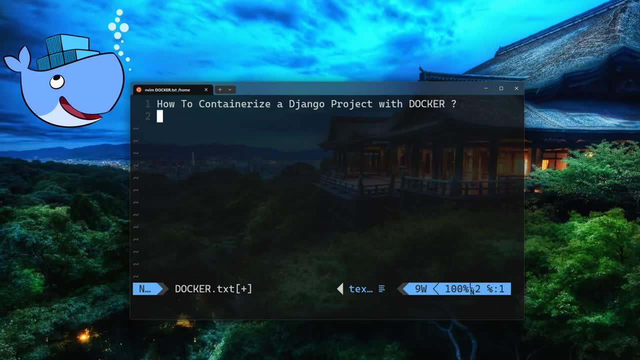 series Docker crash course, But I figured that this topic is still relevant and wanted to share it with you. So the million dollar question is: why should you containerize your apps with Docker? Well, for starters, Docker allows you to package your application into standardized containers. 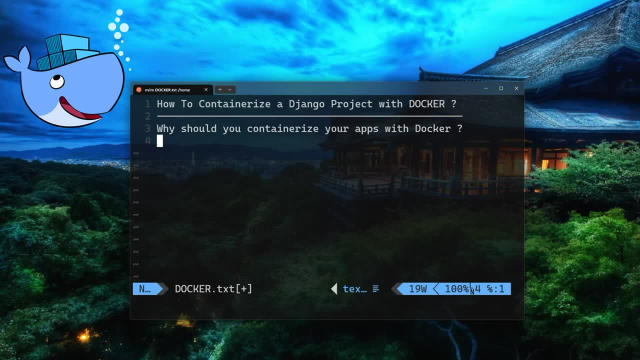 This simply means that your app can run smoothly on your machine, regardless of the operating system or environment. Plus, containers are lightweight and can be easily scaled up or down as needed, And with Docker's tools, you can easily manage containers and automate deployment. But let's not. 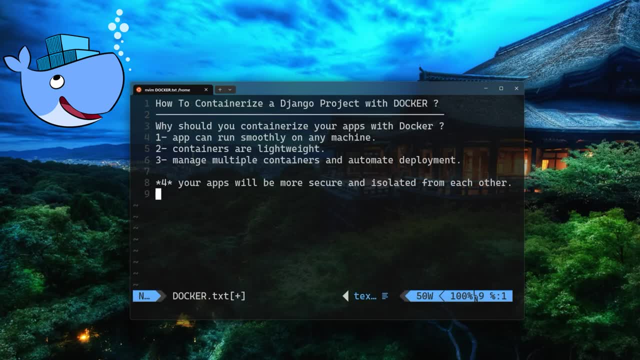 forget about the most important benefit of all: that your apps will be more secure and unisolated from each other. With containers, you can ensure that your apps are running in a controlled environment and avoid any potential conflicts or security breaches. And that wraps up the. 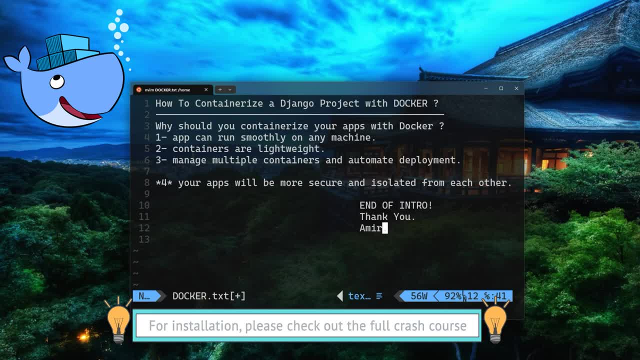 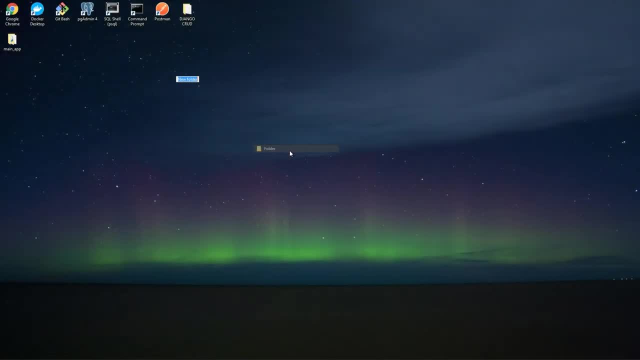 introduction. With that being said, let's go ahead and check out how we can containerize a Django project using Docker. Let's go ahead and create a folder. I'm going to call it Django Docker project. Okay, It's a long name, but just to describe what we're doing, and I'm going to open that with VS. 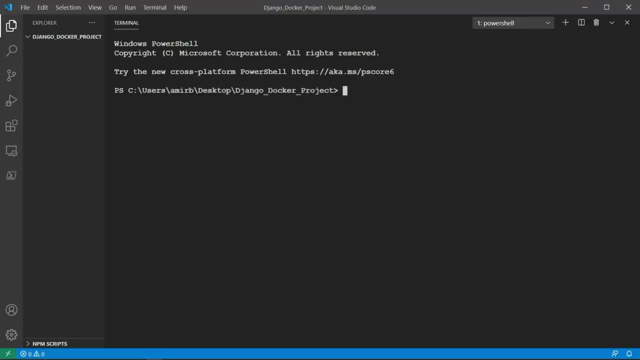 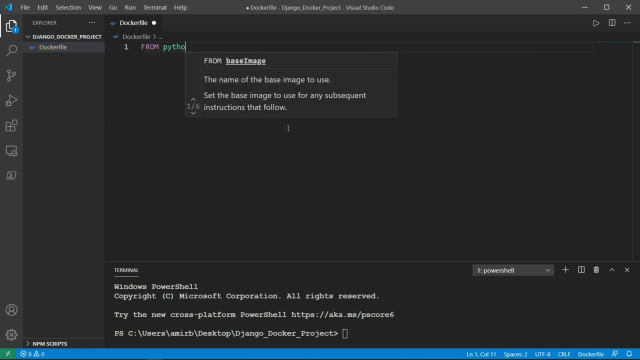 code. All right. So the first thing we need to do now is to create a Docker file. So let's create Docker file. Then we will say: from Python, like we did in the other example, And here we will see together new things that we didn't see in other. in the other example, For instance, we will have the environment. 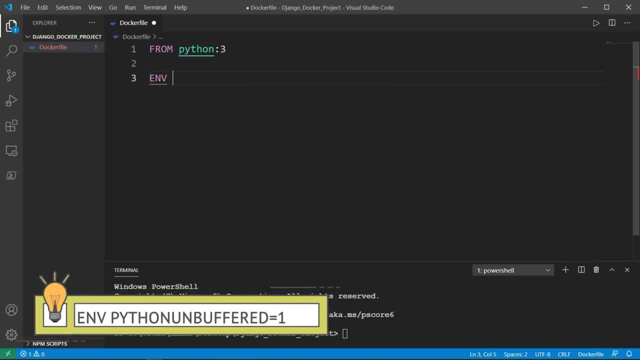 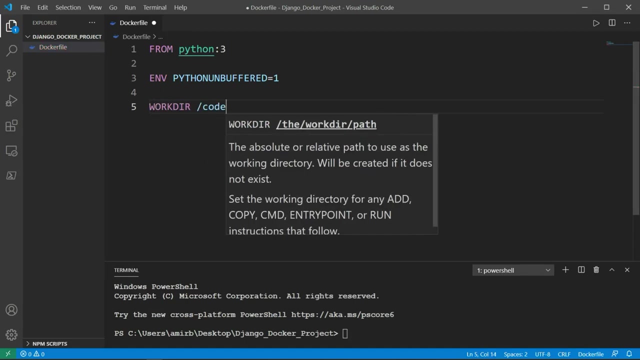 we need to define the environment, And here the environment for Python is called Python unbuffered, And we will set it to one or to true. The next thing that I want is the work directory, which will be equal to just slash code, creating a path or folder called code. Then we want: 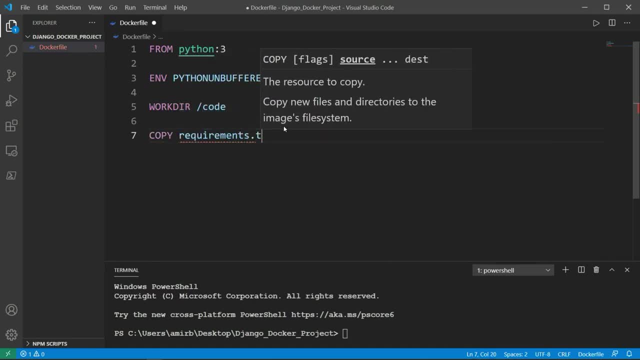 to copy from requirementstxt, which is essentially the dependencies, Okay That your Django project will need. And we want to copy from requirementstxt to the code folder And we will run this by pip: install reading mode requirementstxt. Then at last we will copy everything from the current. 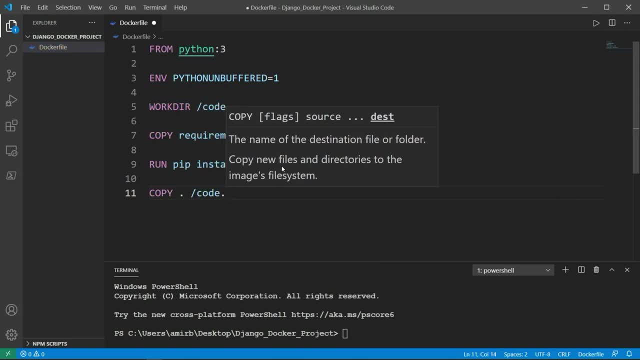 directory to the code folder. All right, And let's go ahead now and create requirementstxt. So I'm defining here the Django version that I want to install as a dependency, And less than 4.0.. Okay, perfect. So now we have saved requirements and closed it. 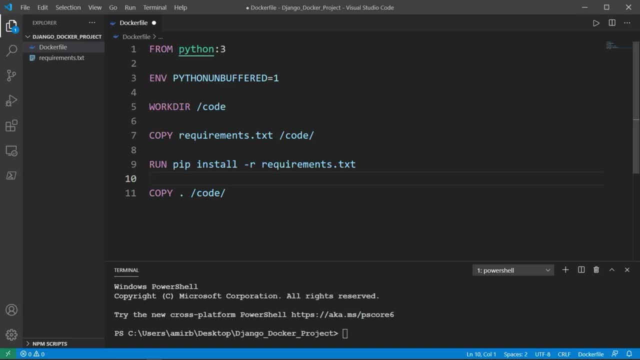 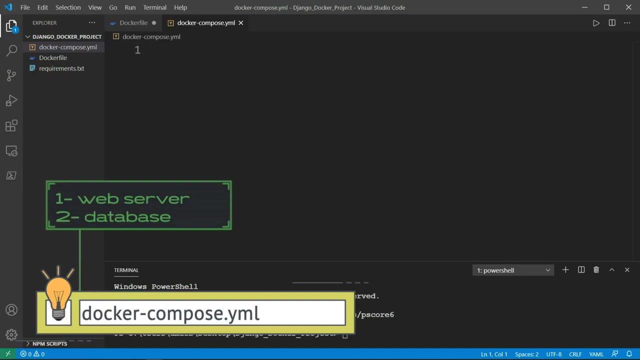 Now let's go ahead and create another important file, and we will call that file Docker dash. compose dot yaml. This file describes the services that make your app Okay. so in this example we have two types of services: web server and database 16, 16. 22.. 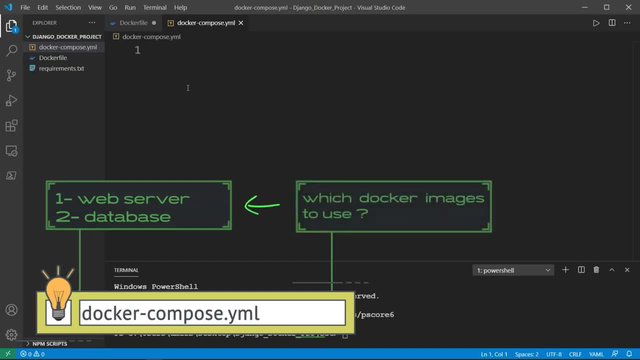 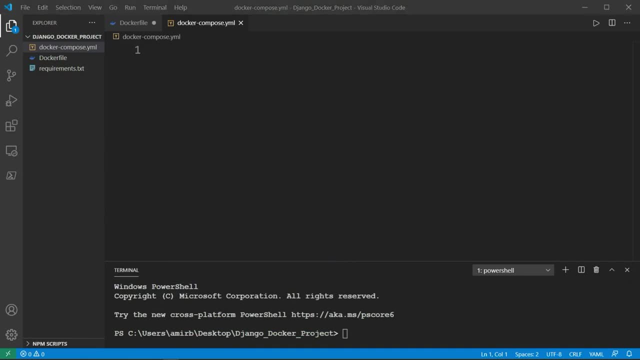 And the compose file describes which docker images these services use and how they linking together. Just for the sake of time I'll just copy that and I will paste it in docker compose. So you can see here we have two types of services: database and web. 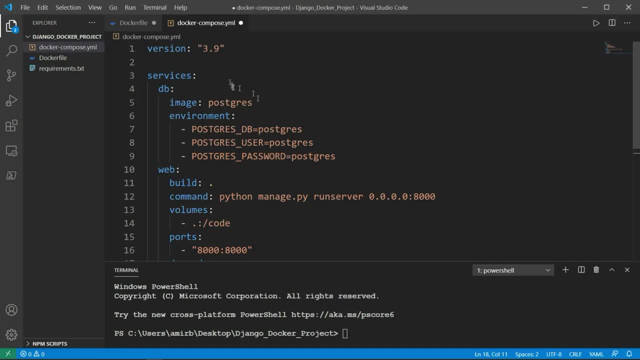 Database is. the image is from postgres, so docker will go to docker hub and will pull the postgres image and install it. Environment: postgresdb equal to postgres, postgres user equal to postgres and the password is postgres. And if you have worked with Django before, you know that Django works with SQLite database. 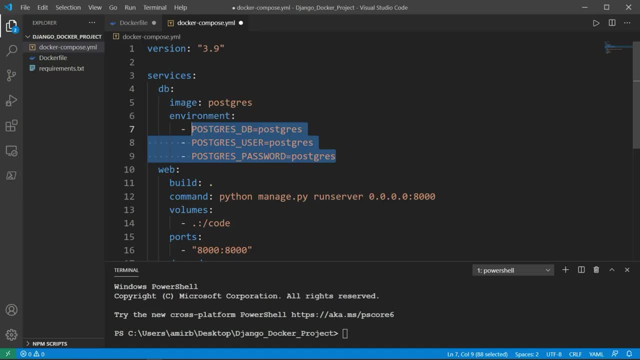 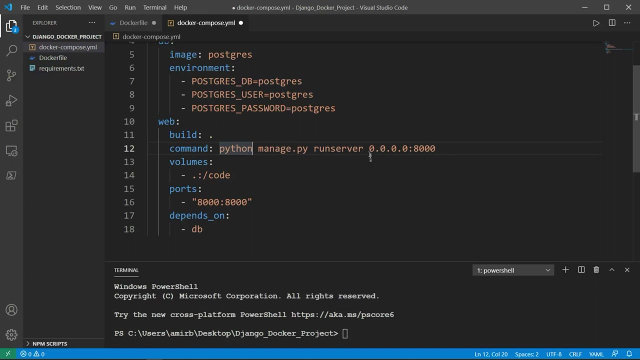 so when we will create our project, we will need to change in the settings file. we will need to change from SQLite to postgres in order to be compatible. Then we have the web build from the current directory command: python, managepy run server 4 times 0, 8000, which is the local host ports. this means that the local port 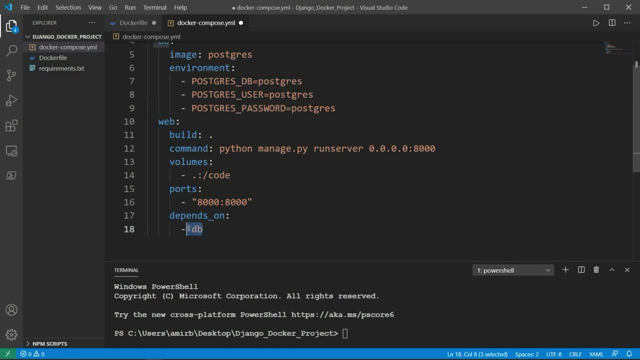 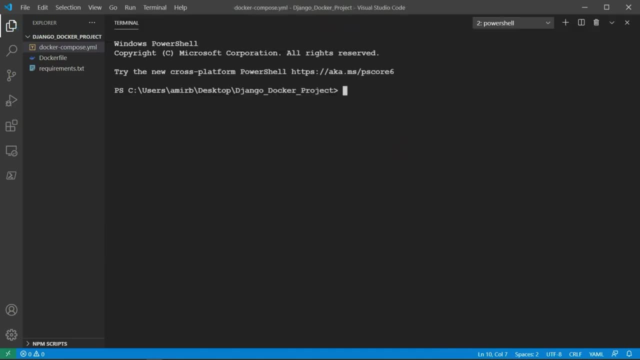 should be set to the public one, and this depends on db, which is set here. Alright, now let's go ahead and create a project. Usually in Django, you would do Django admin start project followed by the name of the project. Here we will do it differently in docker. 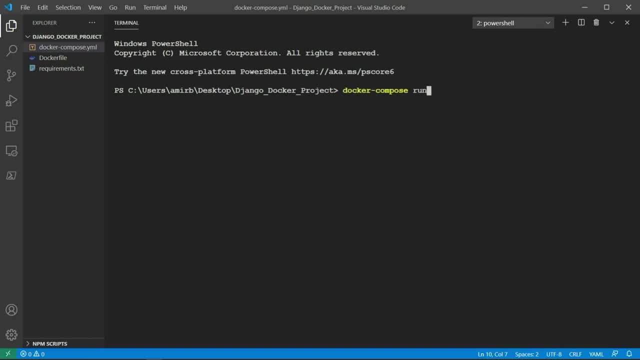 So you will need to type docker-compose, Run web, then Django admin, followed by start project command and the name of the project. So we will say simply Django project, followed by dot, which means I want to compose this project in the current directory. Ok. 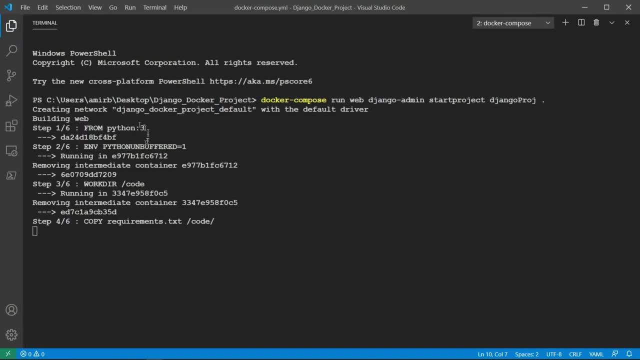 Alright, so it's building from python. you see, it goes line by line in the docker file when we have set from python 3, we have set the environment 316 working directory code, copying the requirements, then installing the requirements. alright, installing Django. 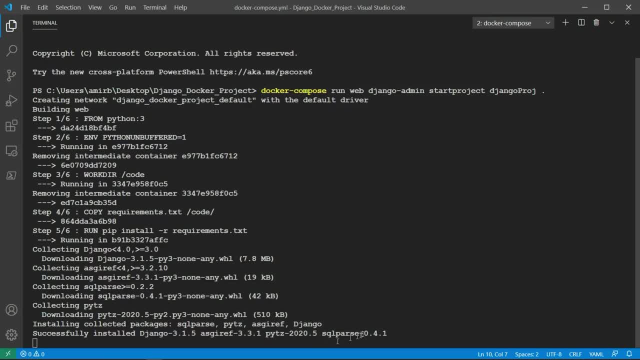 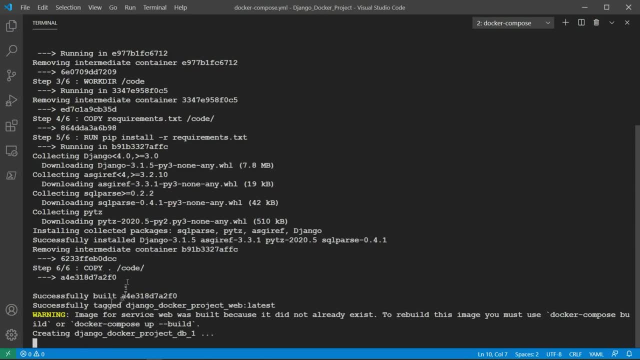 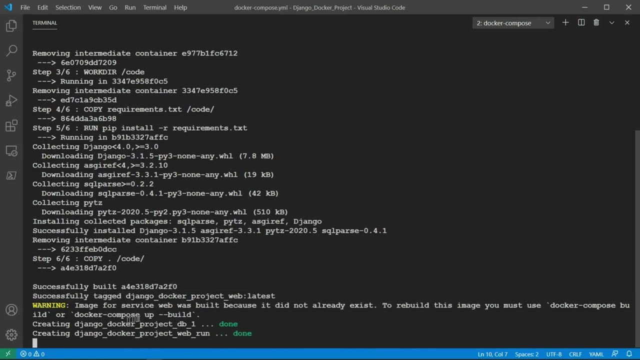 Successfully installed. Ok, Done, Let's call Django. Ok, then copy everything to code. successfully built and this is the image ID. alright, Image for service web was built because it did not already exist. To rebuild this image, you must use docker-compose build or docker-compose up. dash, dash build. 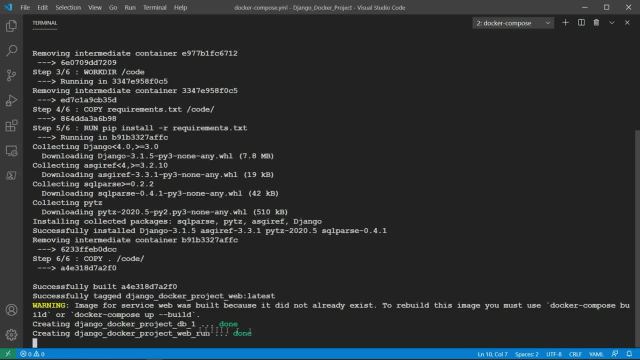 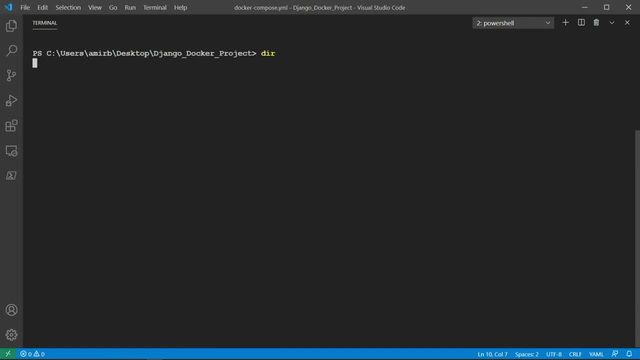 We will see that later, Alright, Ok, Perfect Now, if we will dir what's inside our Django docker project, we will find that we have successfully created the Django project. We still have the docker-composeyaml, the docker file requirementstxt and managepy. 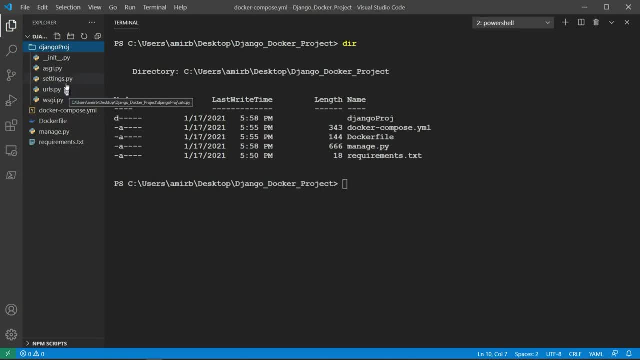 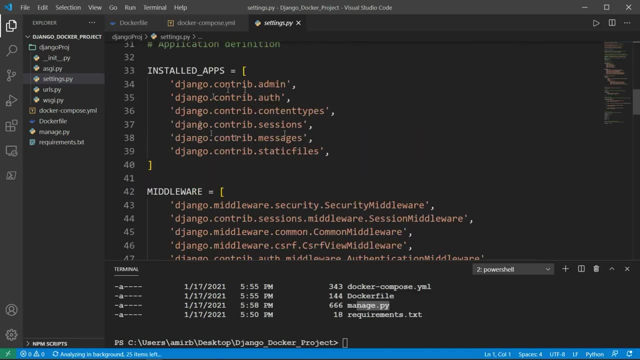 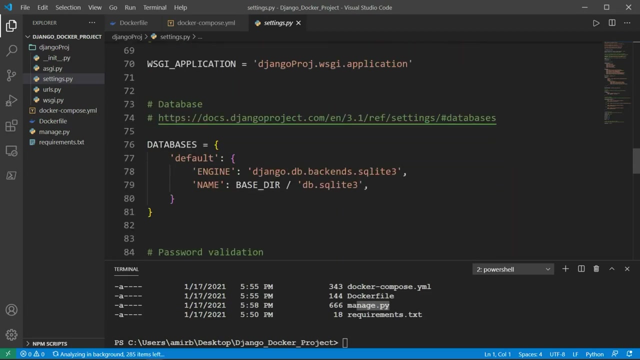 Ok, So we have our Django project and let's go ahead and change in the settings. we will need to change the database and later we will need to add the name of the application in installed apps after we will create it. Then we have the database. 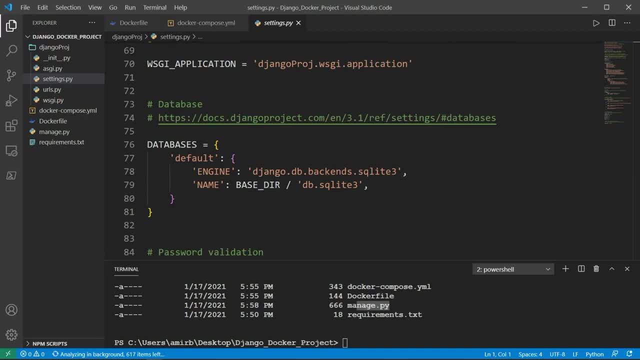 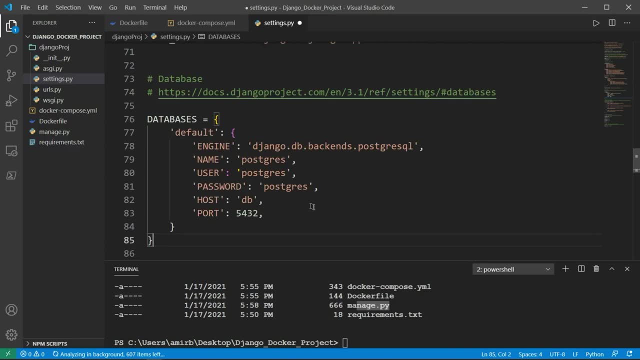 This needs to be changed, alright. So, also for the sake of time, I will copy it and I will replace with the Postgres OSDP. the port is 5432.. The engine is 643.. Ok, The engine is backendspostgresql. ok. 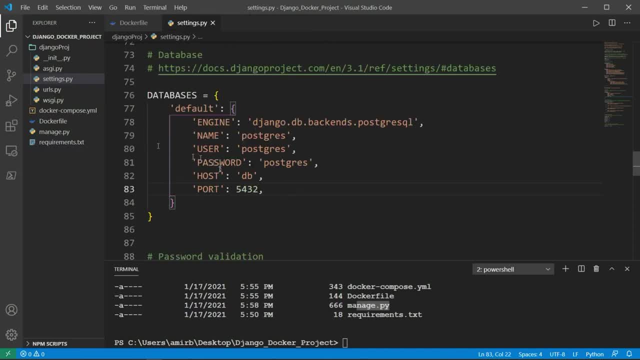 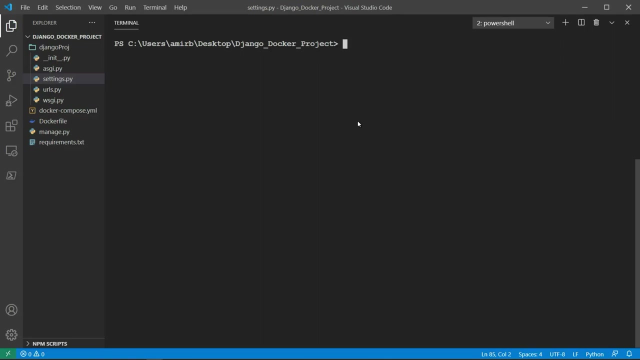 And now we have a compatible system between the settingspy and the docker-composeyaml. Alright, let's close that. let's close that And let's get back to our terminal. Now let's go ahead and run our application from docker. So we will run the docker-compose up command. 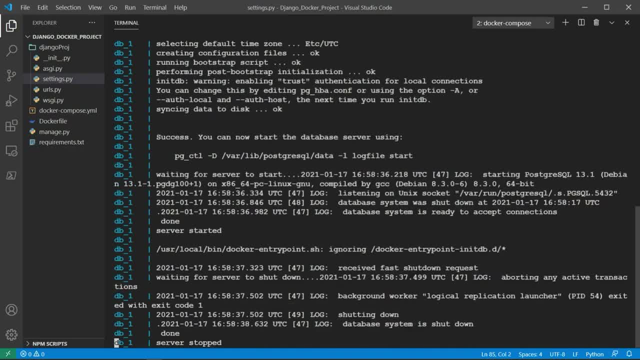 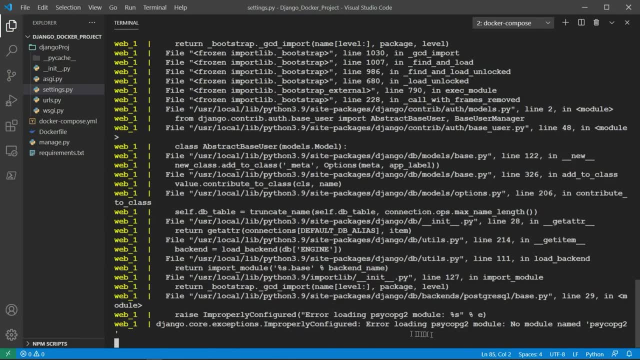 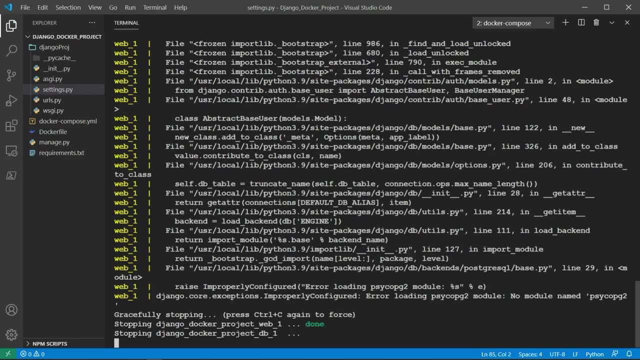 And we will hit enter. Ok. So we have got an error loading psycho-pg2 module: No module named psycho-pg2.. So we will need to add in our requirements the psycho-pg2 module. So let's exit docker. ok, stop in Django, alright. 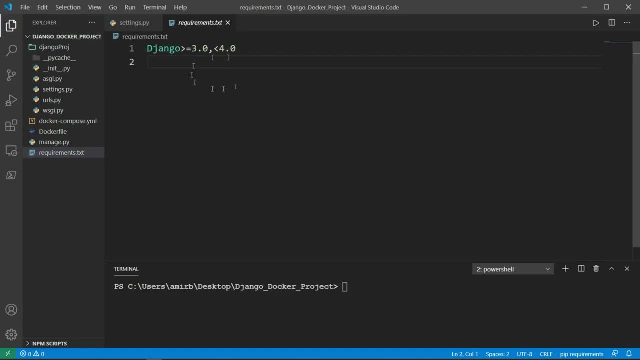 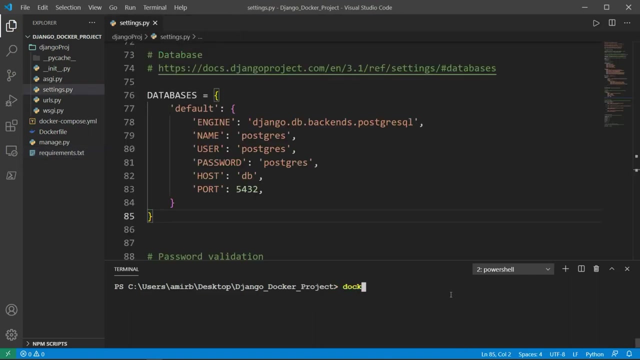 And let's go to requirements and add the psycho-pg2 module, So psycho-pg2-binary version 2.8 plus. Ok, Let's save that And let's docker-compose build in order to update what we have done. Ok, 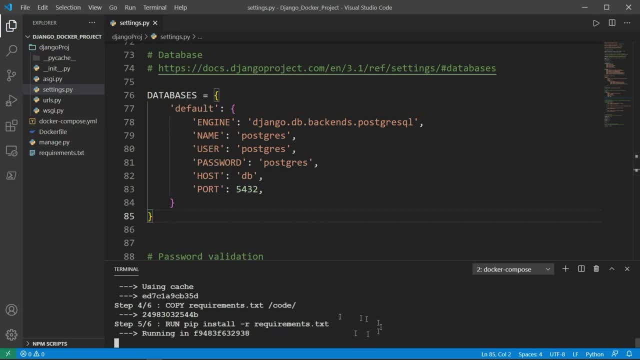 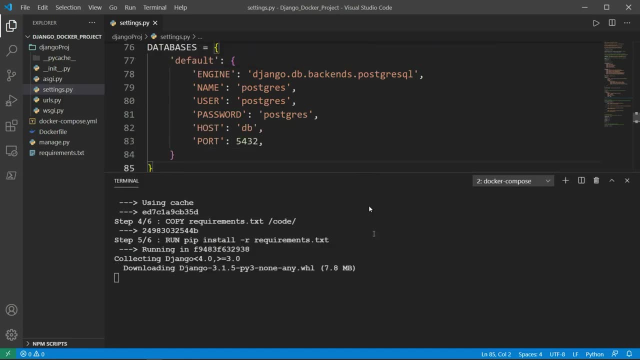 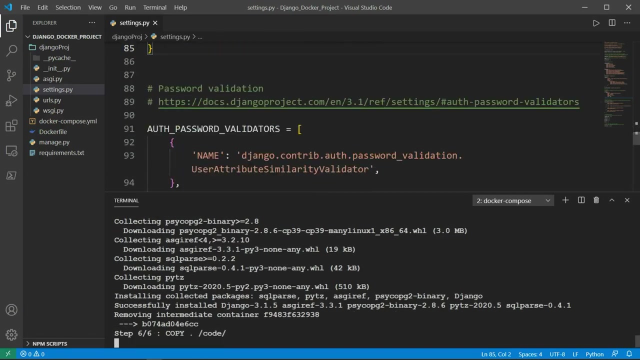 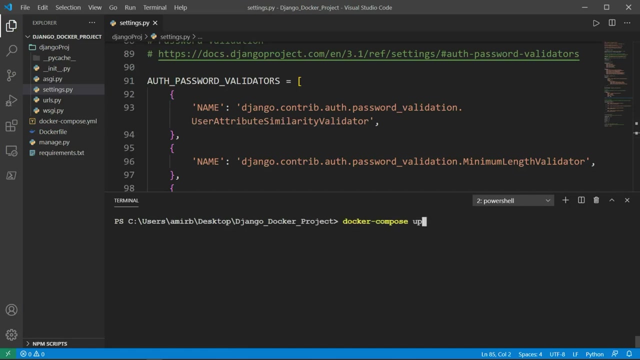 So every time you make some changes, you need to update that in order to be reflected in the docker image. Alright, so collecting and downloading psycho-pg2, and once that done, we will actually try to run again the server from docker. So let's say docker-compose, up to run the project inside docker. 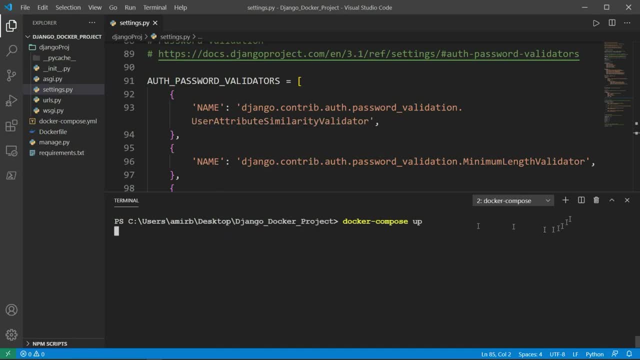 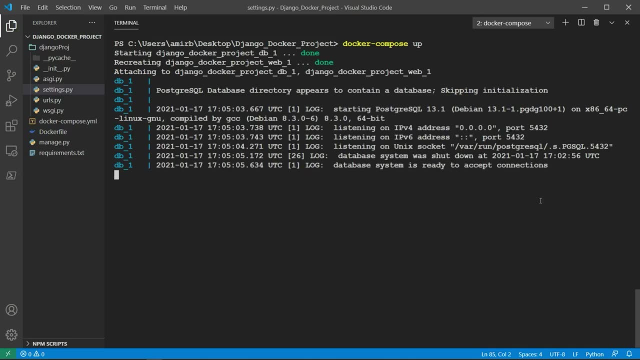 Ok, Looks fine, Ok, perfect. So starting development server at four zeros, 8000, which is the local host, Let's go ahead and click on that. Let's open. Ok, perfect, So it's working. Ok, so it's listening on port 8000, and this is running from docker. 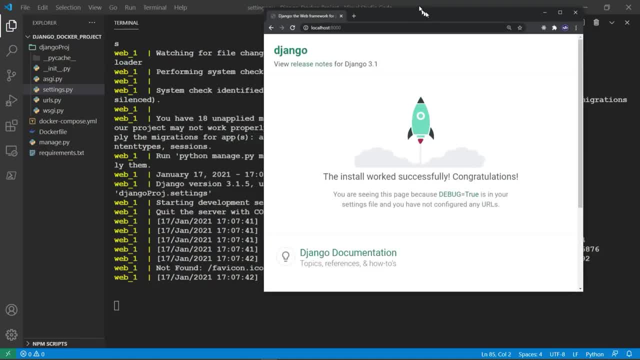 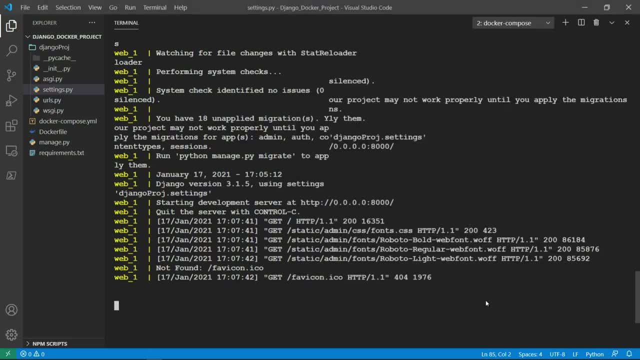 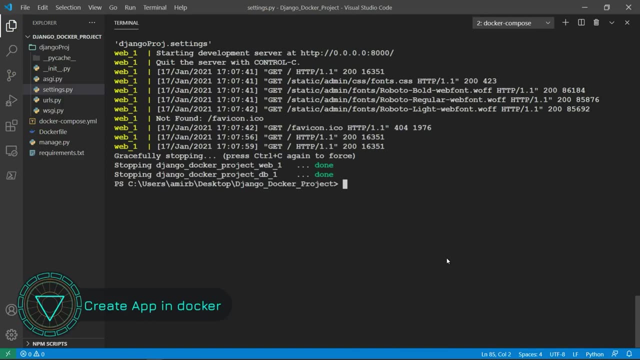 This is not running locally from a machine. Ok, So let's close that and let's hit control C just to stop the server. So the last thing that I want to do in this course is to create an app for the project, And to do that is very similar to what we did in the previous course. 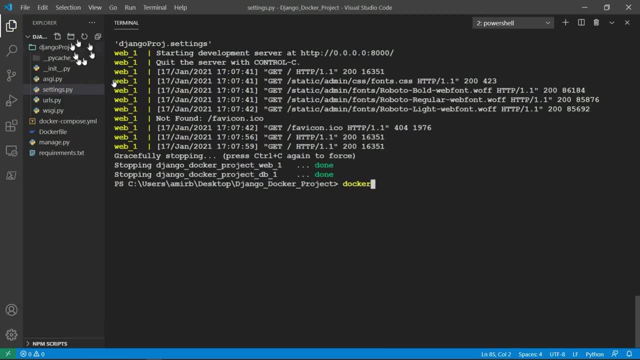 Ok, So that is very similar to what we did to create the project. So docker-compose run web. Then we want python managepy start app and the name of the app. Let's say I love docker, And here you don't have to make a dot. 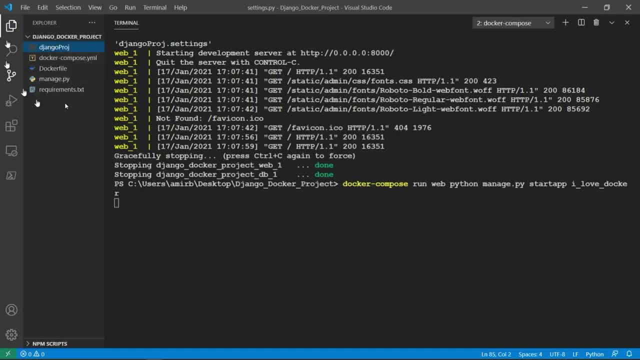 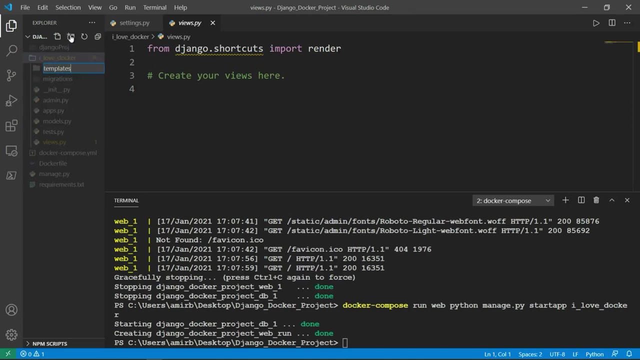 Just hit enter and it will be created in the directory. Alright, perfect. So we have- I love docker created, So let's go ahead and make some modifications. First of all, I would like to create templates, And in templates I will create indexhtml. 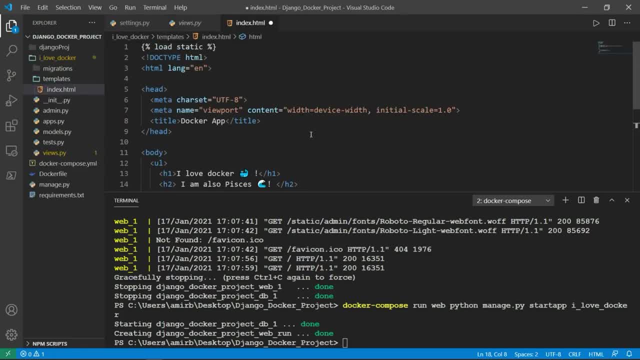 Ok, And I will, And I will just paste that. It's just simple boilerplate with two tags. I love docker. I'm also piscus. Alright, Just nothing fancy really. And I want to go to views And I want to create index function. 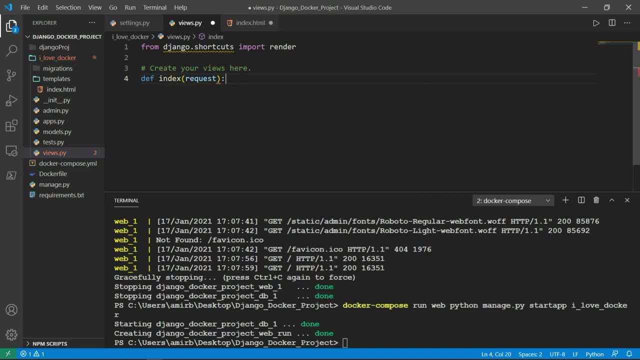 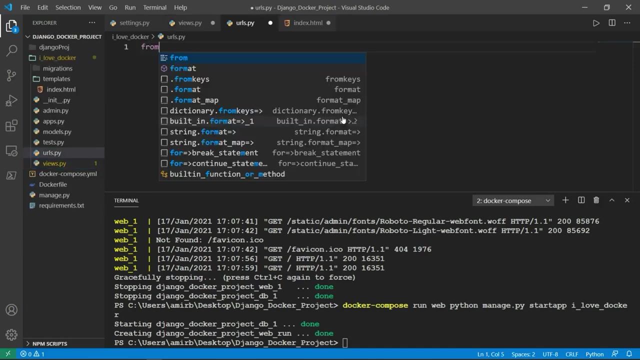 And it takes a request, Alright. And what it does? it returns render And the request and the file is called indexhtml. Ok, Alright. So this is views Also in. Also here I would like to create urlspy And from djangourls I want to import the path. 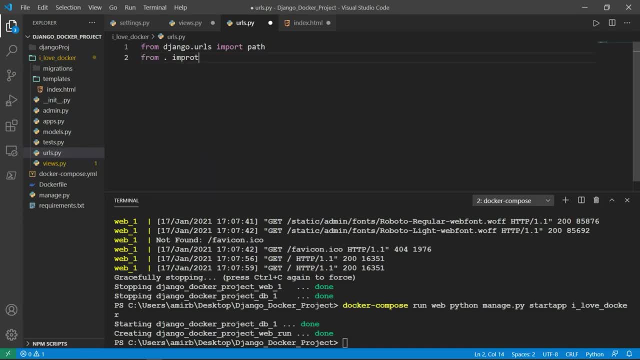 And from current directory I want to import the views And the patterns. URL patterns: Ok. Viewsindex: Ok. So the path is when it's empty path or just a slash. I want to go to views and just trigger the index function. 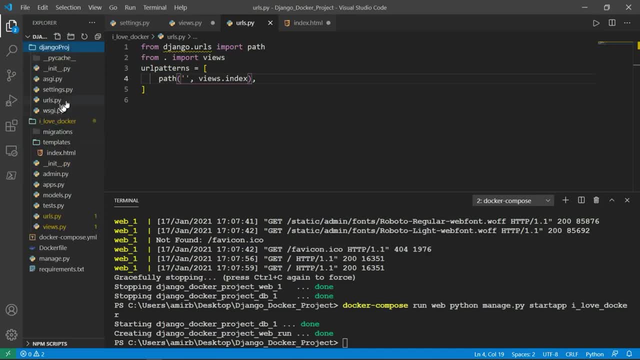 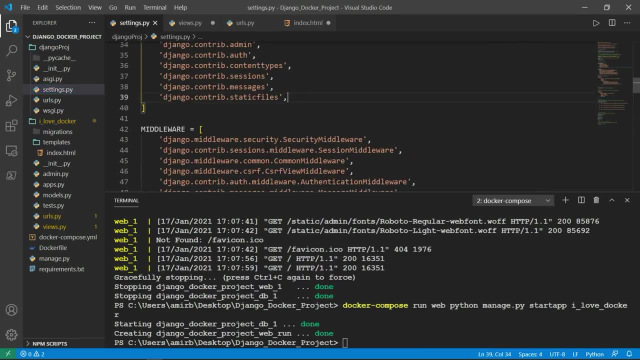 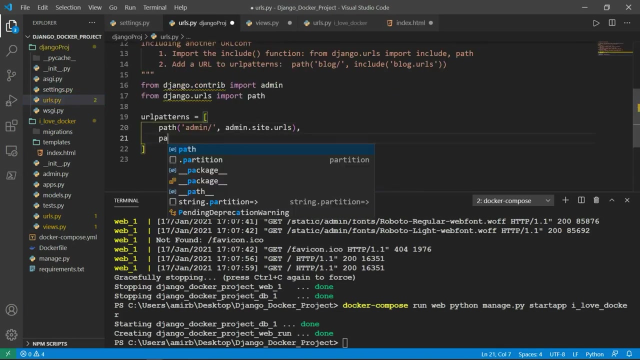 Alright. Now in the django project itself, I would like to add that app in installed apps. Alright, So come here, Add i underscore love, underscore, docker. And also in urls. I want to add the path, which is empty string. It goes to: i underscore love, docker, dot urls. 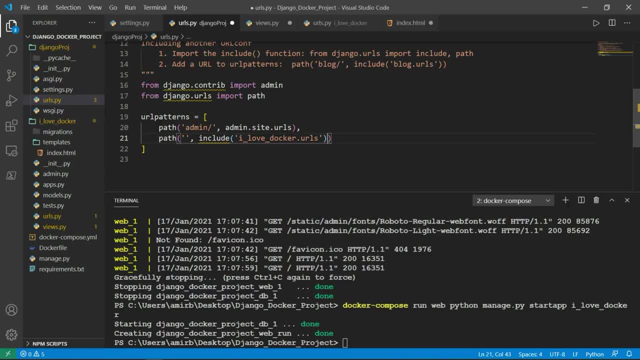 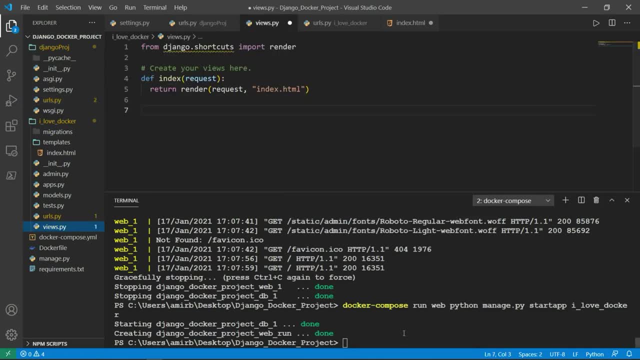 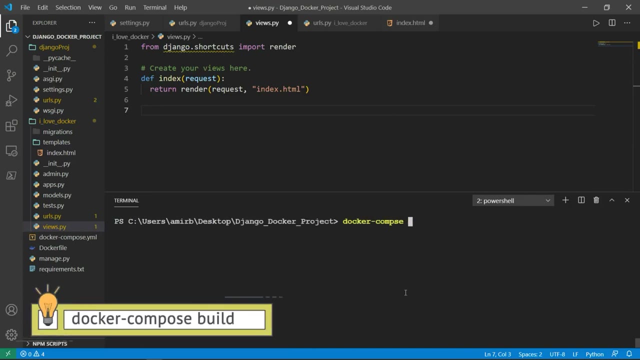 Alright, Ok, Nice, And I want also to import include: Ok Now, in order to update, we will use the command docker compose, build to update, But as we want to run the application from docker after updating, I can use a shortcut for that. 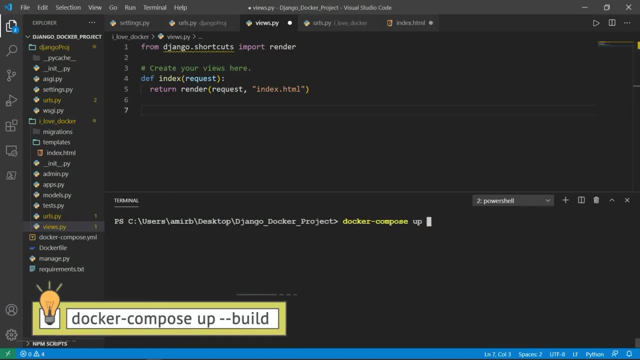 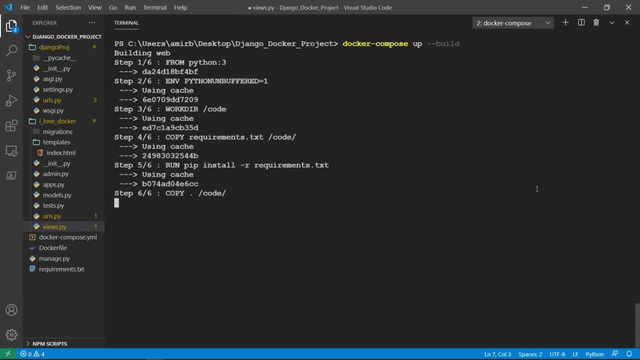 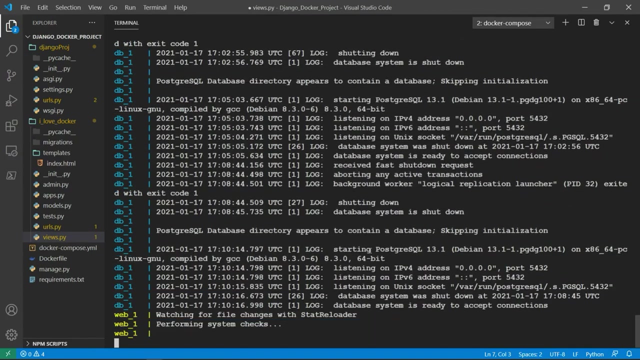 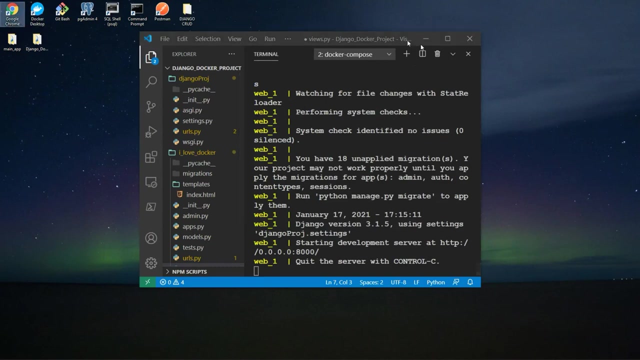 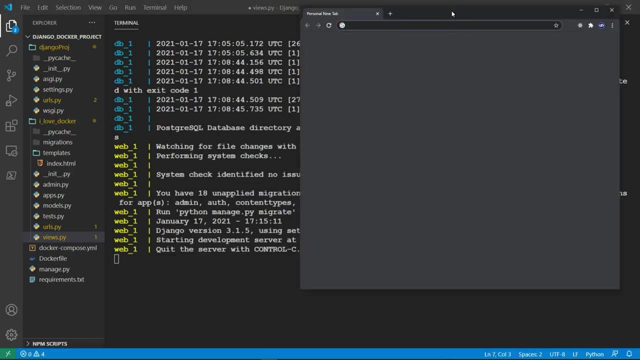 So I'll say: docker, compose up dash, dash, build. So it finished building. It checked for any changes, Successfully built, and give us this image, This image id. Alright, Ok, Perfect, So looks ok. Let's go ahead now and open the browser to check out the local host for our program, which is working from docker. 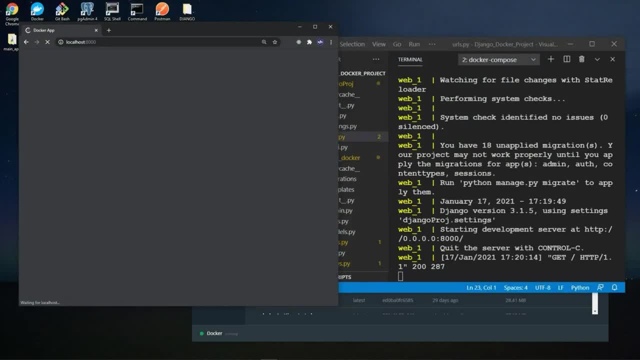 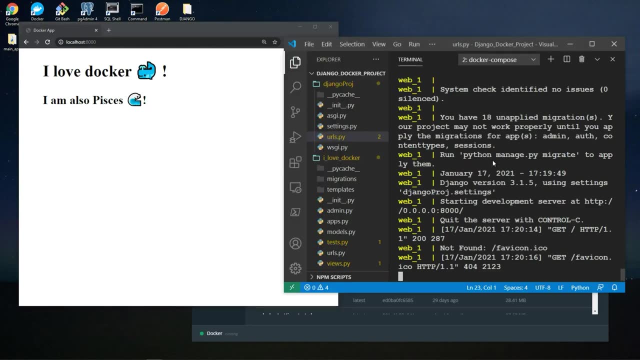 Let's go ahead to local host port 8000.. And we have. I love docker. I am Piskus. So we have successfully created a Django project And we have created also an app, And this app is running from docker. Alright, guys.